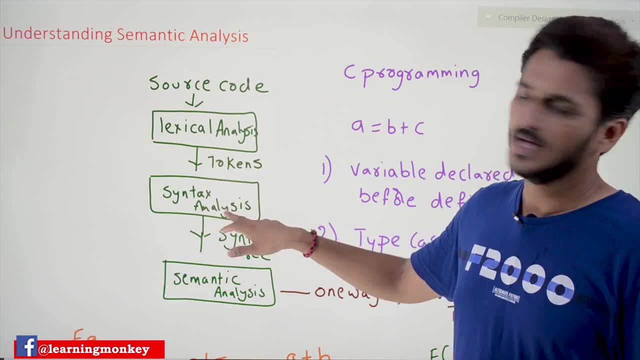 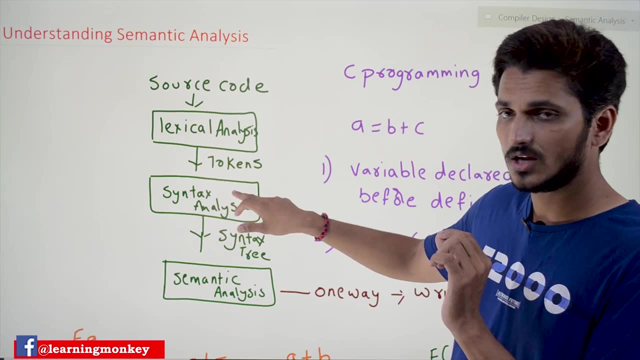 These tokens are taken as input to the syntax analysis phase. These tokens are taken as input to the syntax analysis phase and it is going to identify syntactically correct or not And it is going to give the syntax string. This is the output for the syntax analysis. 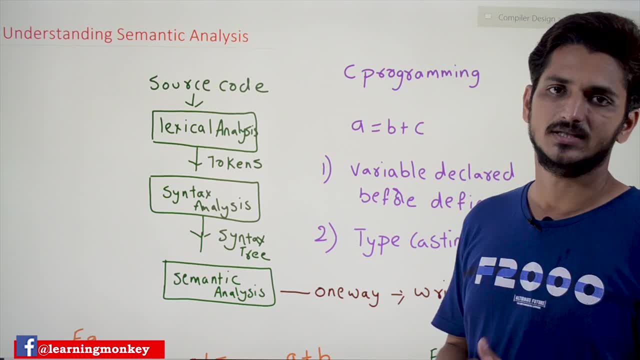 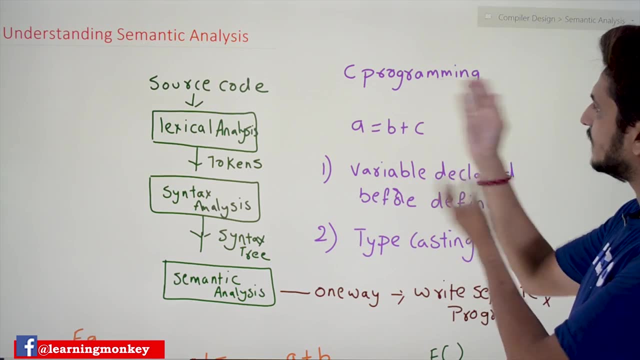 This is taken as input to the semantic analysis phase. Let's try to understand what we are going to check in semantic analysis phase. We are taking C programming language. If you are going to check for, A is equal to B plus C expression in C programming language. 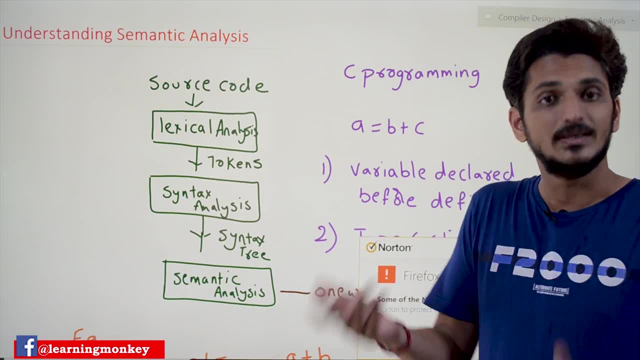 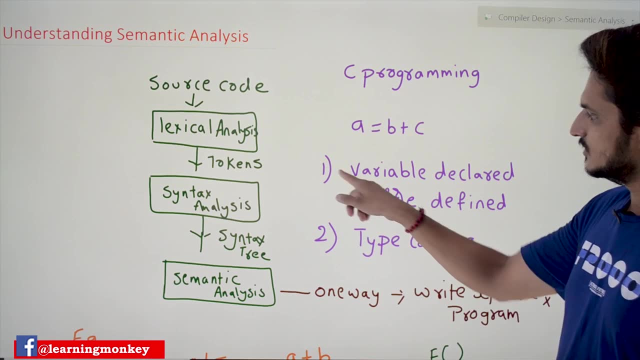 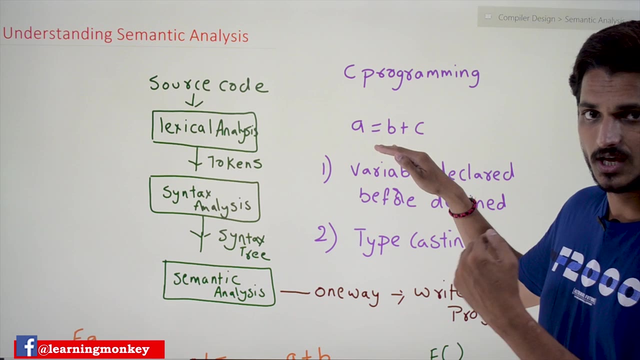 You can take any language. Each language has its own semantic conditions. Let's try to understand what's the conditions we have in our in C programming language. So first of all we are going to take C programming language. So first one is, whenever you are going to check the syntax whether the statement is syntactically correct or not. 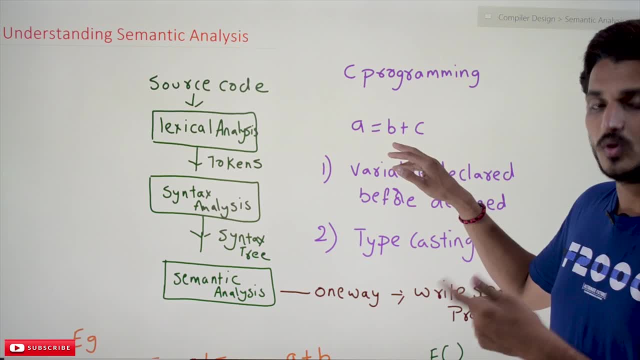 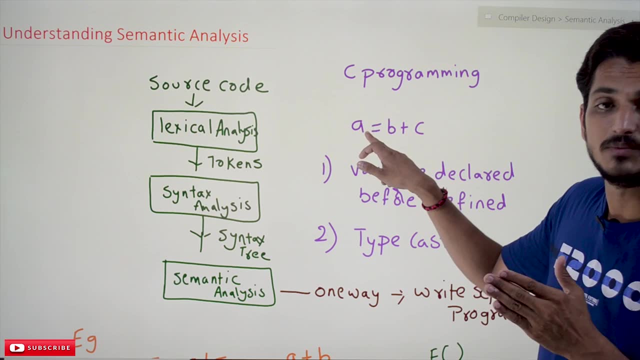 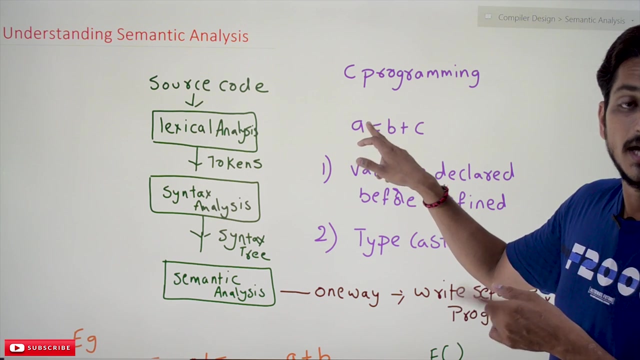 Then we need to check one more thing also: What's that? we have written some conditions for C programming. What's those conditions? If you are assigning a value to a variable A, before assigning means, before defining the value, before defining A, It should be declared. 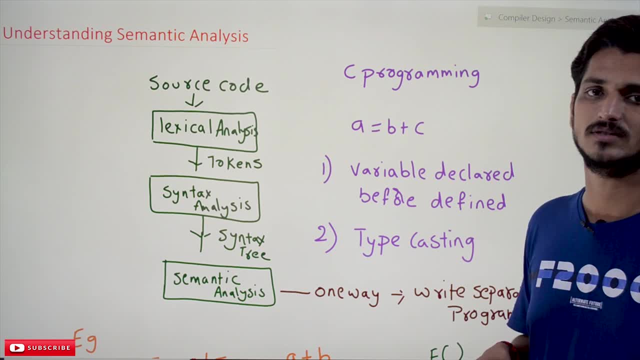 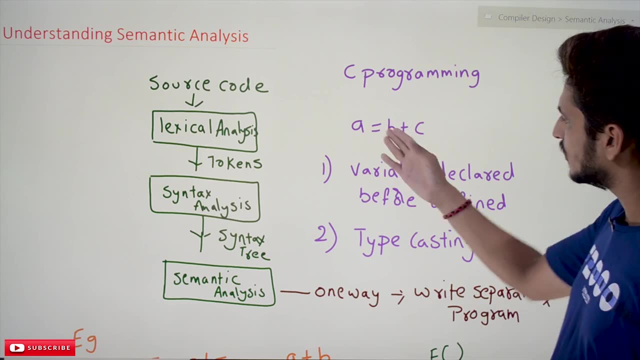 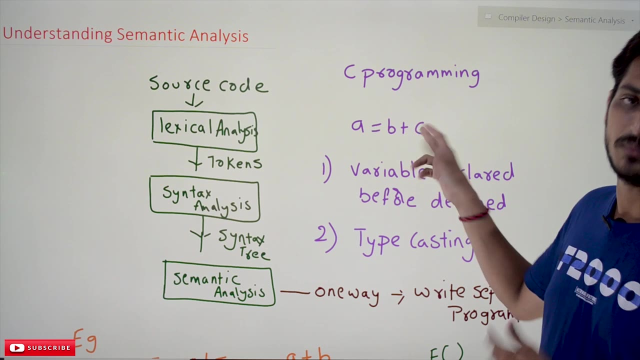 That is the condition we have to check in C language. This condition is not there in Python. So based on the programming, language, conditions changes. And one more thing: variable should be declared before defined. The second thing is type casting. If you are doing some action, B plus C, both are having the same type or not. 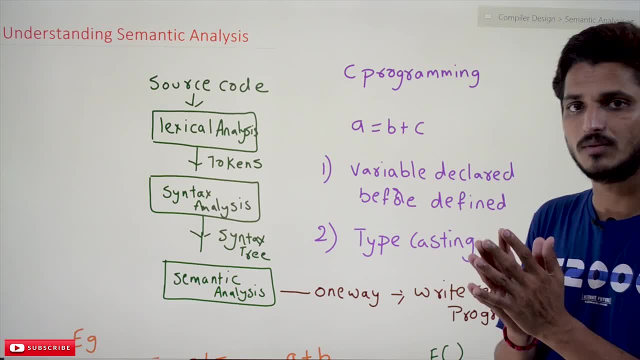 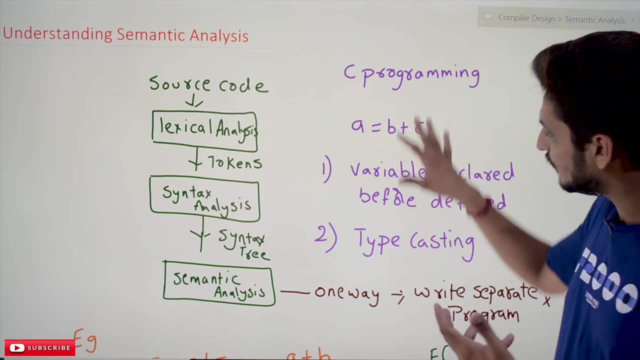 That is what we have to check. Otherwise we need to do some action based on the types that present for these two variables. So we have to do some actions. in C language These type of conditions comes under semantic analysis. This is called semantic analysis phase. 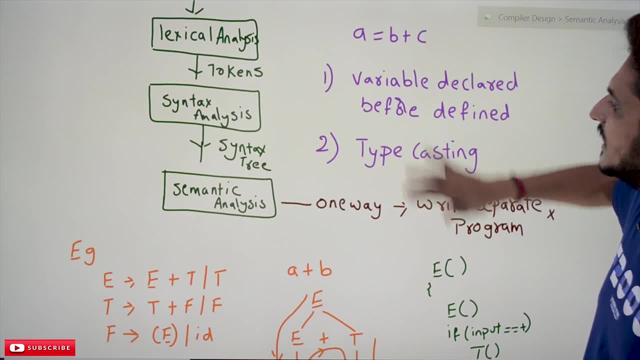 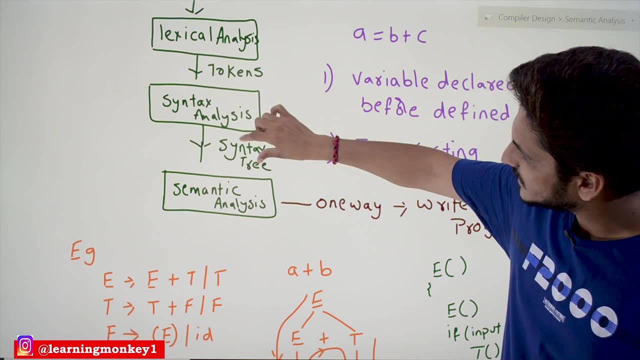 So now, in order to do the semantic analysis- one way we can do that- Take the syntax tree. that is the output that we got from syntax analysis phase. as input to the semantic analysis- We need to write a program and check the semantic conditions. 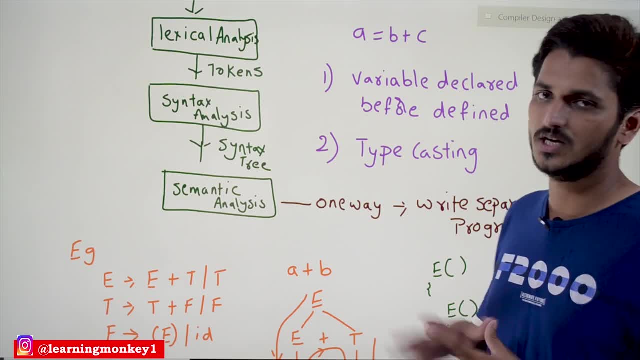 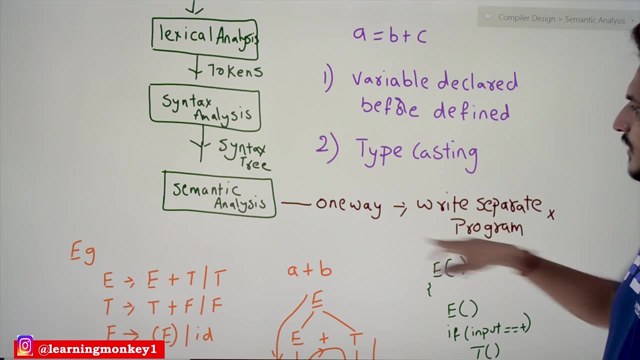 This is one way, but most of them will not follow these conditions. So this way, So this writes. So one way is. One way is writing separate program. We are writing a separate program. No, we don't write a separate program. 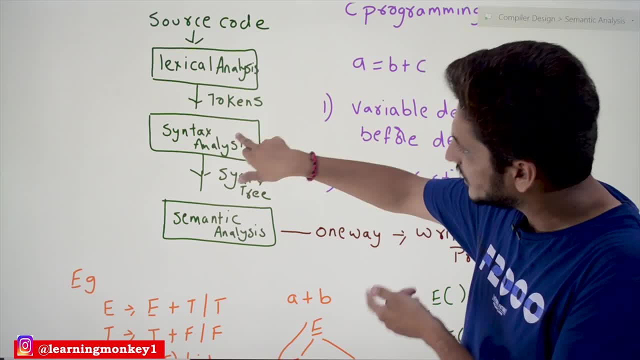 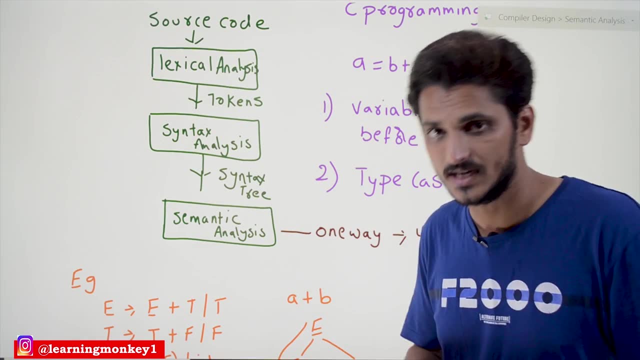 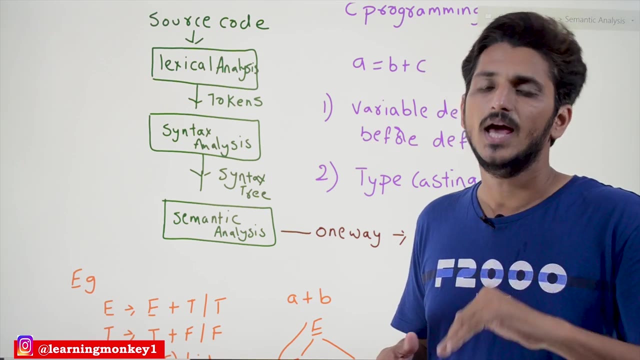 Based on the whatever program we have written in syntax analysis phase. During the execution of syntax analysis phase, we are going to check the semantic conditions also How we do that, How do we write the program? That understanding will be provided in this class. 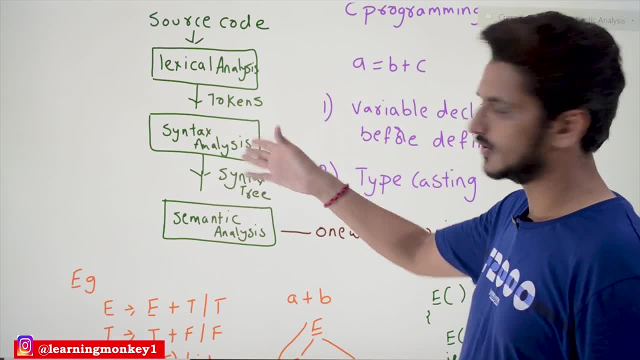 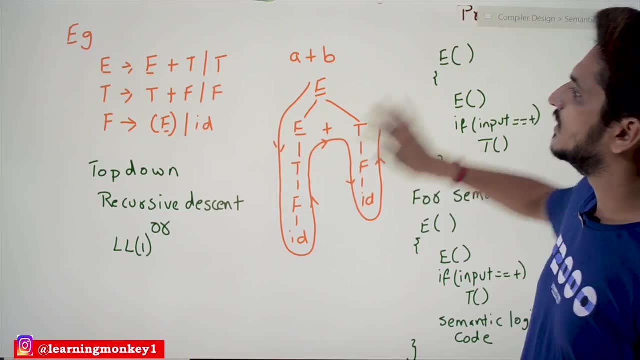 In our next class we will do some examples How we do that and what are the conditions, How we write the conditions, All those things. So let's take an example. This is the basic grammar which we are following in our previous classes. 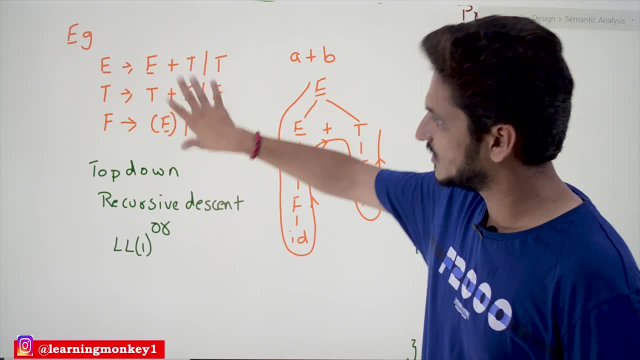 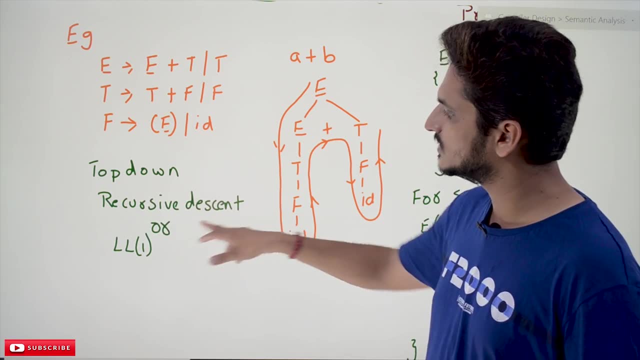 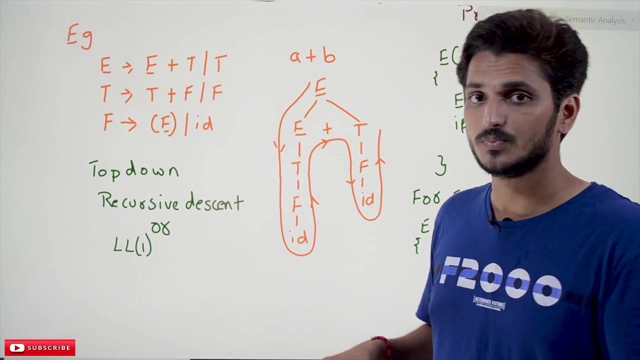 The same grammar we are going to take. e tends to e plus t. This is the expression grammar If you are following top down approach. We discussed two top down approaches, that is, recursive descent or LL1.. You take any program whenever you are finding to evaluate the syntax of the expression. 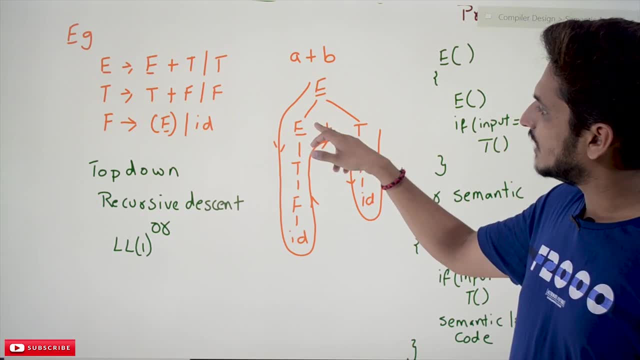 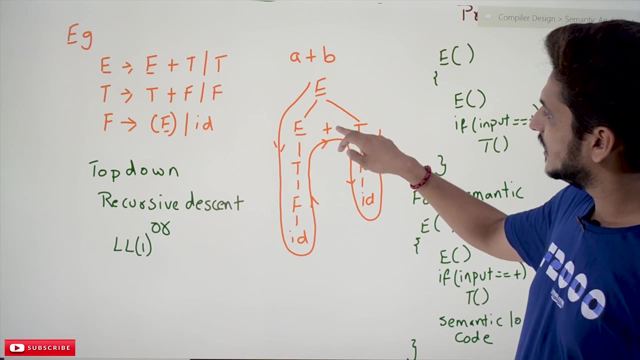 Let's take an expression: a plus b. e is going to evaluate in top down approach. e tends to e plus t. e is evaluated t, t tends to f, f is id, Then it is going to check for plus, Then it is going to expand t. 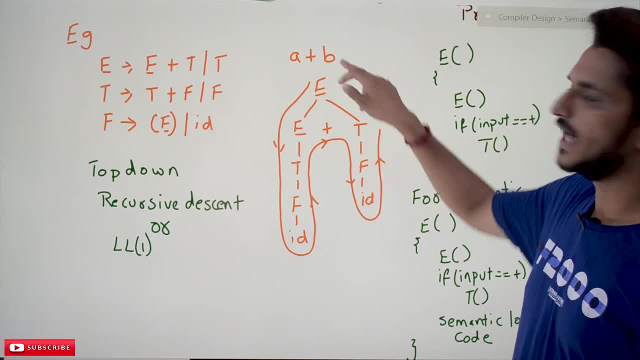 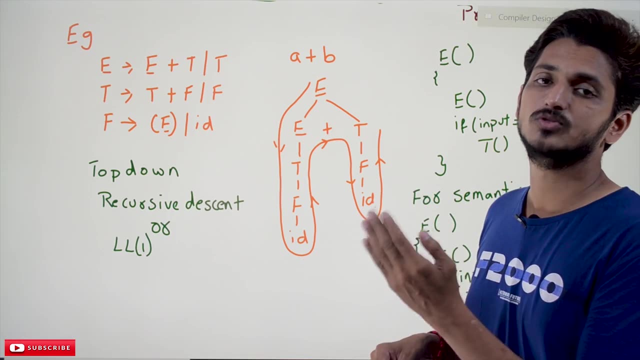 And it is going to check for id. Then a plus b has been identified. How it is going to expand Left. most derivation tree is going to get in top down approach. So when it is going like this, This is how it is going to evaluate. 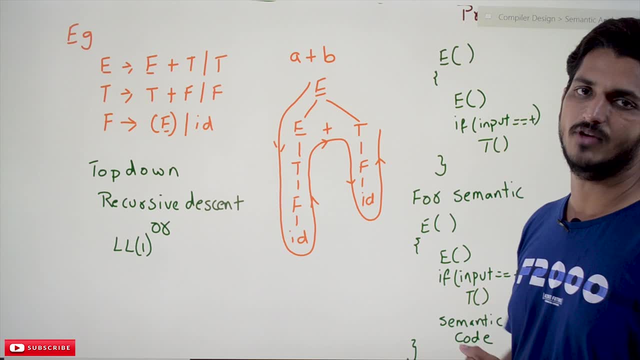 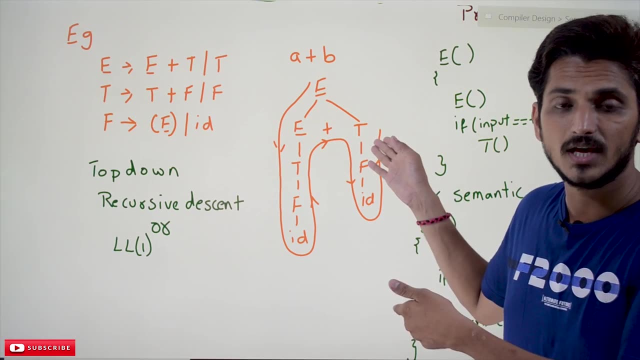 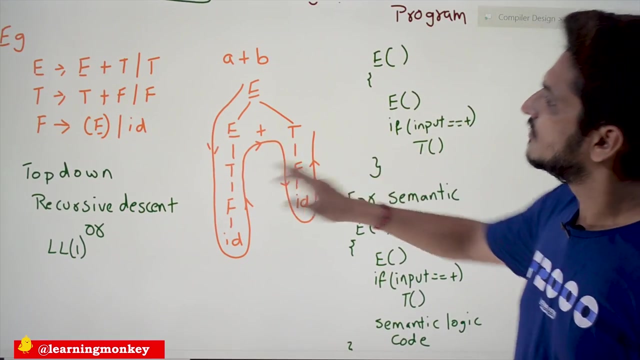 Expand. Expand the x context free grammar that is given. So whenever this e plus t, this production has been finished. Yes, you can write the code here to check the semantic conditions How we write that. Let's take this For this grammar. if you are following recursive descent parsing: 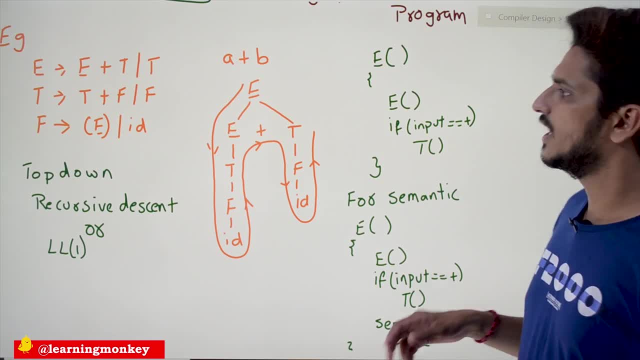 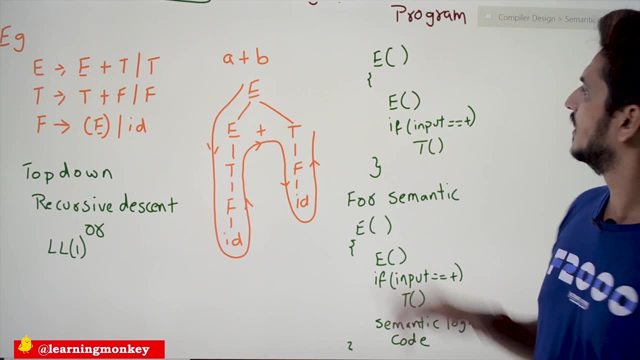 How we write the code in our recursive descent parsing technique. For each non terminal we are going to write a function. E is a non terminal. That's why we have written a function for e. E is going to call e of. if input is equal to plus, then call t of. 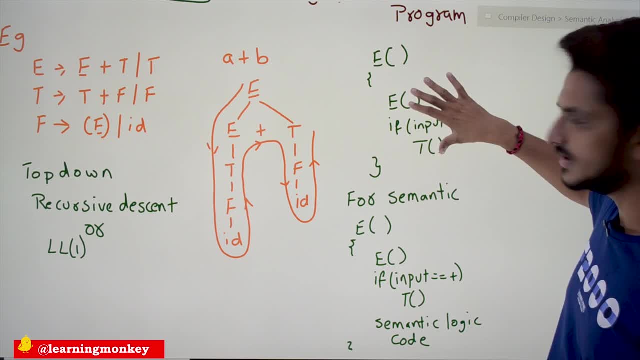 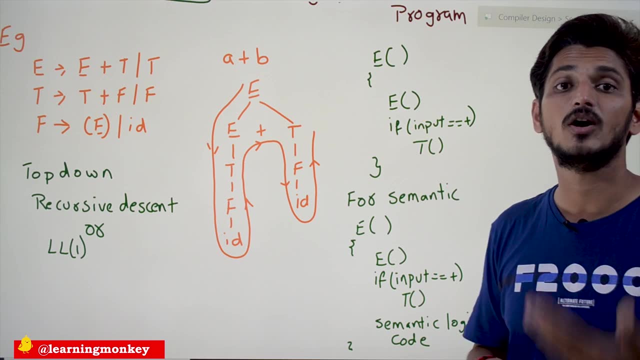 t of is a function, So this is the function. This is the body of the function for e. After completion of this function. Yes, here you can write the semantic logic. Is it compulsory to write the logic after completion of this function? 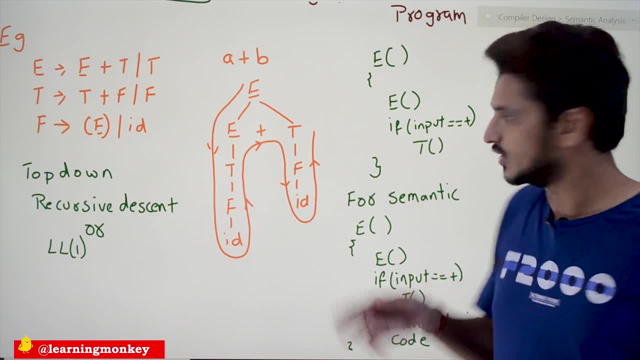 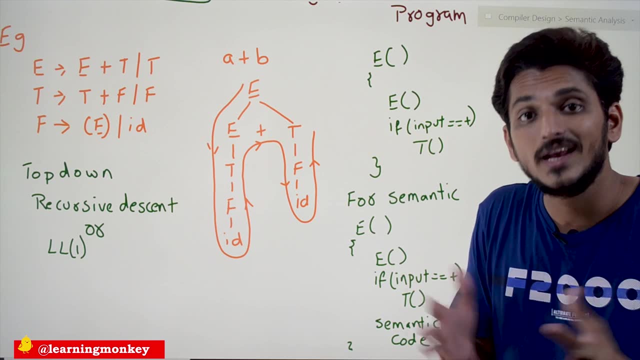 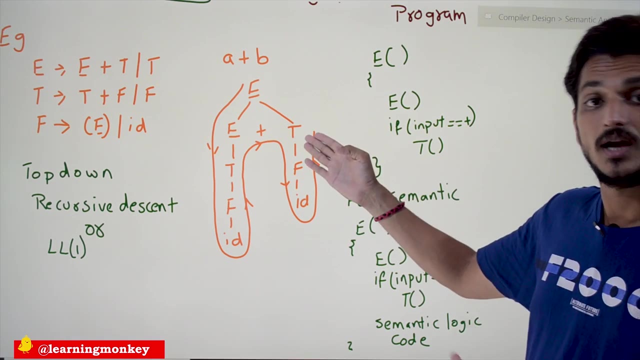 No, Wherever you want to check, You can write. after checking the if condition, You can write. after calling the e function, You can write the semantic logic according to your requirement. In this example, we are going to check the type casting of two variables. 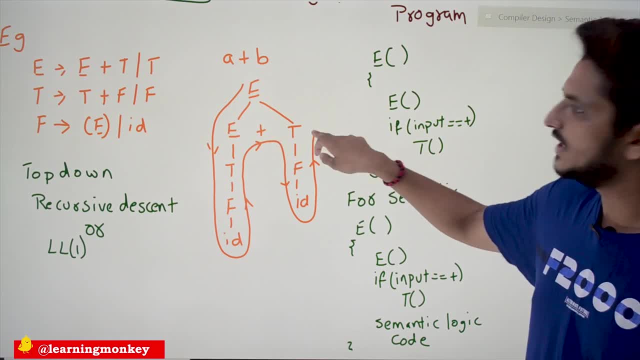 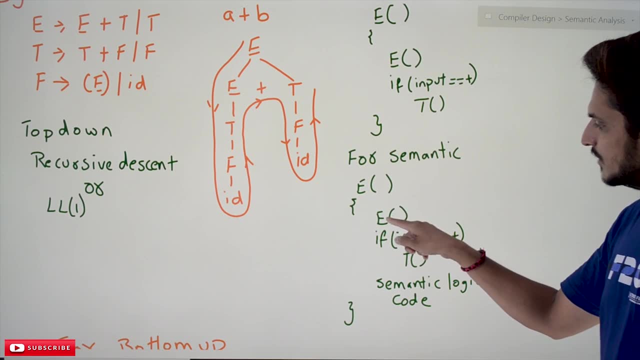 After completion of this evaluation: e plus t. So that's why we will write like this: e of the same code. We are adding the semantic logic. So, after completion of e of, if input is equal to plus t, of is called. 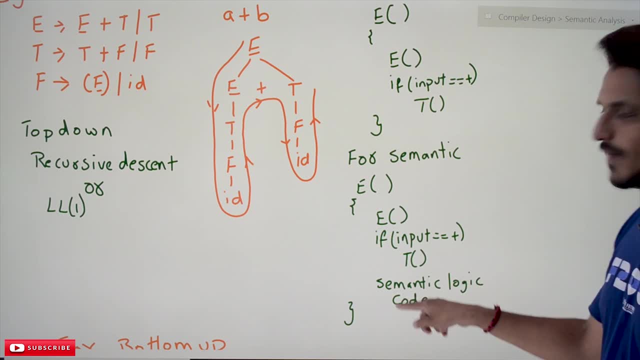 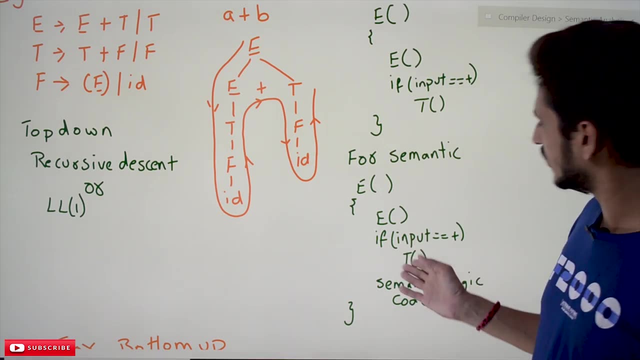 After completion of t, After coming out of: if We are going to check the semantic logic code Should be written here. So this is how we will write the code, Not only like, Not only in checking the semantic conditions, The same way we can. 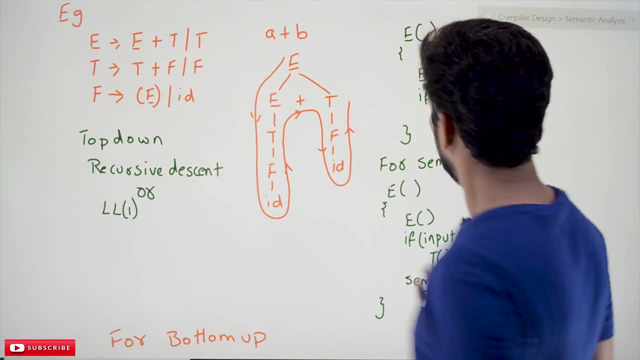 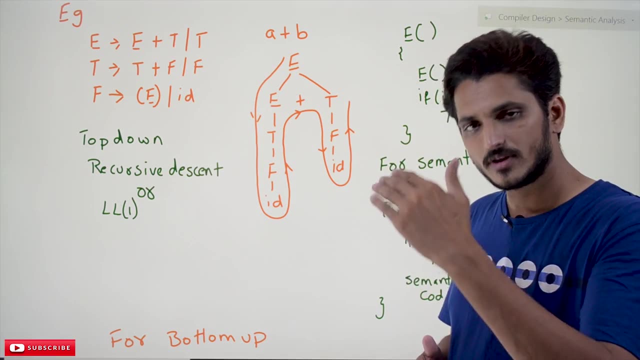 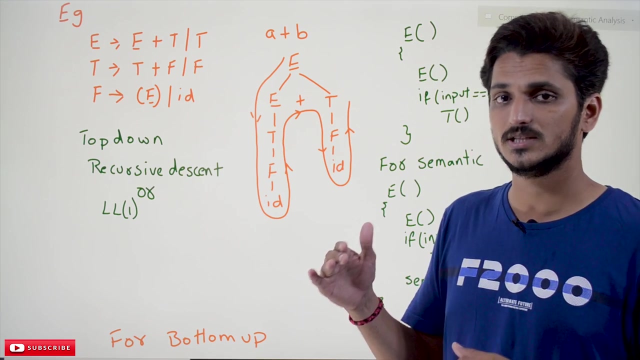 The same way Whenever we are discussing about the phases of compiler. First lexical analysis phase, After its semantic analysis- No Its syntax analysis phase. Then we go with semantic analysis phase. After that we are going to check for three address code. 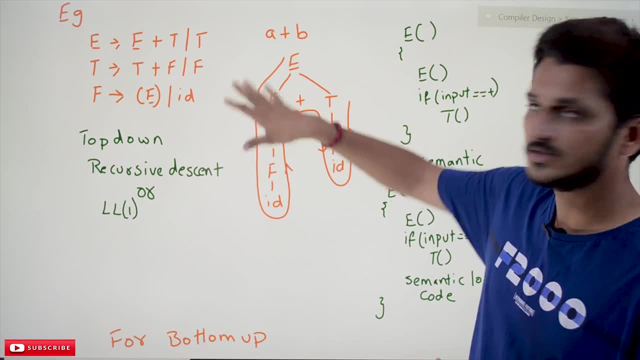 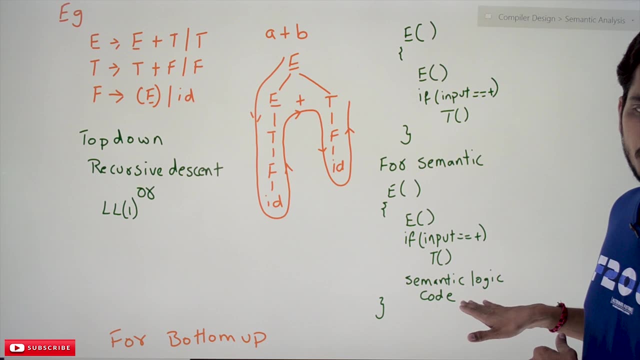 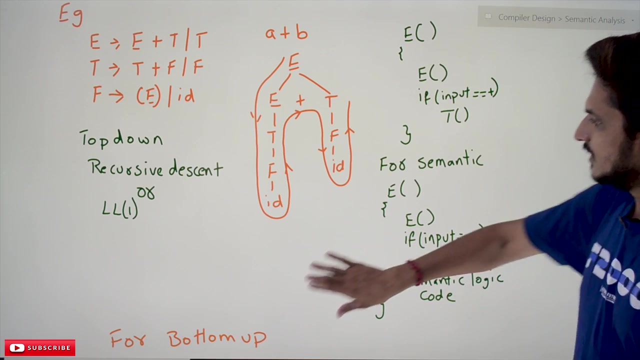 We are converting our analysis into three address code. You can write the code here to convert our program into three address code also. These points are very important to understand our next classes. So this is how we write, Not only in top down approach. 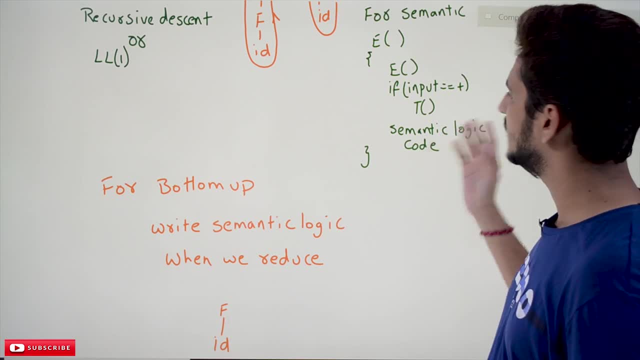 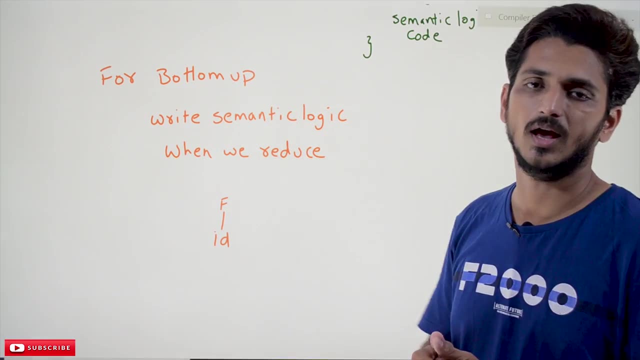 You can write this: semantic conditions, even in bottom up approach. So writing semantic logic: when we are going to reduce the action In bottom up approach, We are not going to expand, We are going to reduce. During the reduce action, You can write the logic. 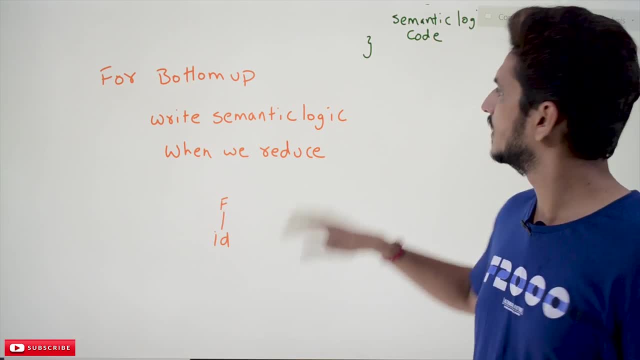 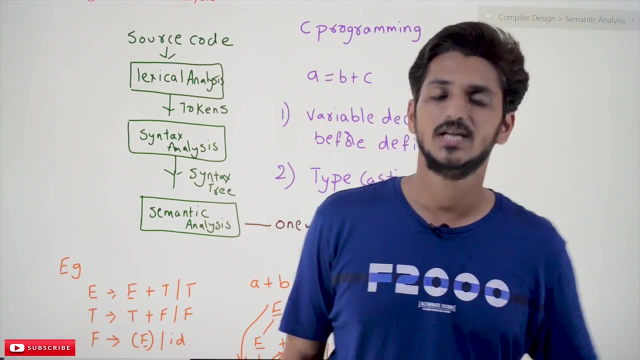 Whatever the way you want to write the logic, You can write that logic here. So this is the basic understanding for semantic analysis. In our next class we are going to discuss in depth understanding about semantic analysis. Hope you understand the concept. If you have any questions regarding the concept, 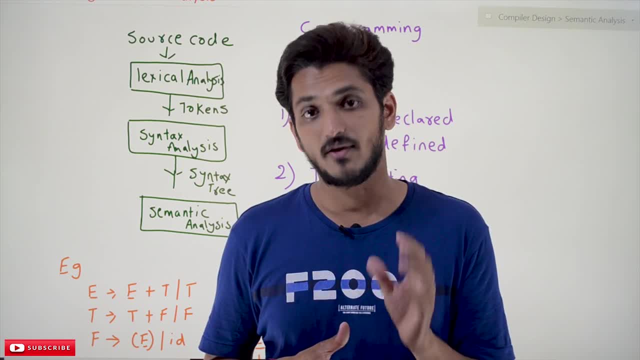 Please post your questions in the comment section below. Thanks for watching. If you haven't subscribed to our channel, Please subscribe to our channel And press bell icon for the latest updates. Thank you.